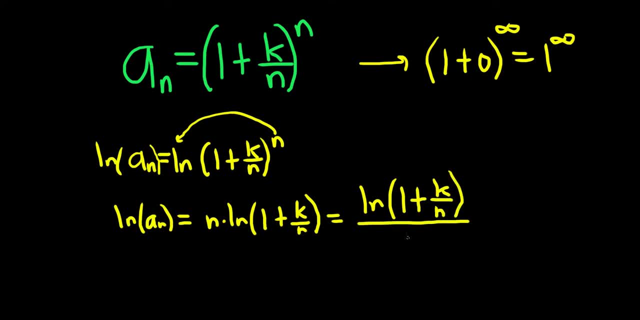 over, and then you write it as one over n. And the reason that you do this is because now, if you take the limit, if you think about it, you're going to get the n to the infinity. and then you're what's happening here In the numerator, you'll get ln of 1, right, because k over n approaches. 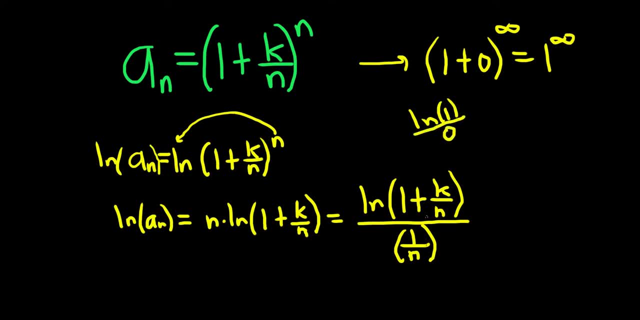 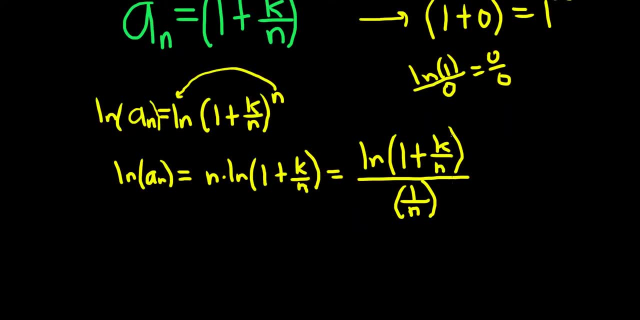 zero In the denominator, you'll get zero right, because 1 over n approaches zero. So ln of 1 is zero. So you get zero over zero. So you can actually use L'Hopital's rule, which lets you. 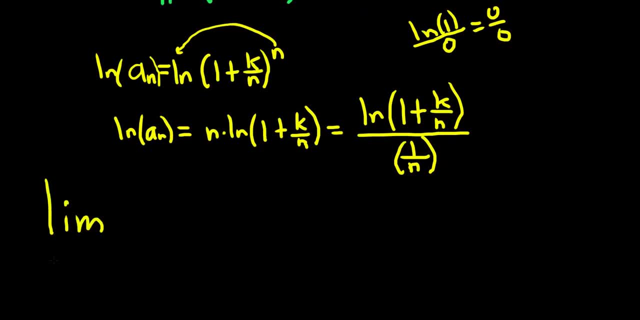 take the limit. So let's go ahead and take that limit. So the limit, as n goes to infinity of the natural log of a sub n, is equal to the limit, as n goes to infinity of the natural log of 1 plus k over n over 1 over n. 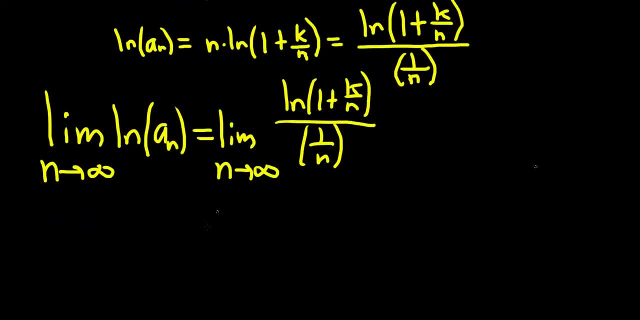 Okay, and this is equal to the limit as n approaches infinity of a sub n. So you can actually take that limit as n goes to infinity of the natural log of 1 plus k over n over 1 over n. Okay, so now we just have to take the derivative of each piece, because this has the form. 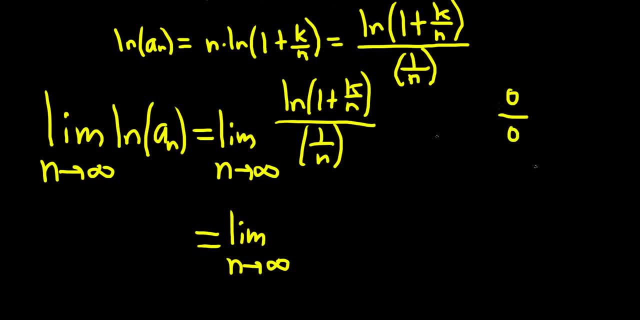 zero over zero. Again, ln 1 over zero is zero over zero. So we can use L'Hopital's. So the derivative of ln x is 1 over x. That's from before. If you have ln x and you take the derivative, you get 1 over x. So here it's going to be 1. 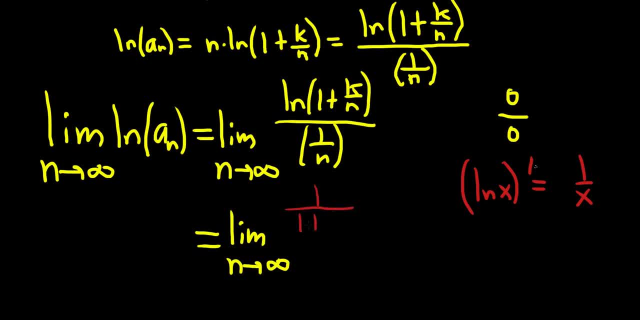 over 1, plus k over n over n. So you get 1 over x. So here it's going to be 1 over n over n over n, 1 plus k over n. that's like your 1 over x times the derivative of the inside. so we're thinking of: 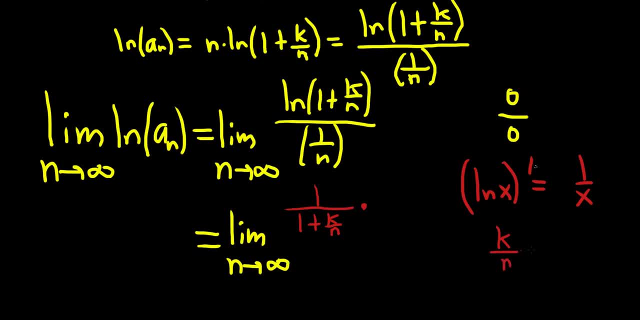 k over n and we're taking the derivative. pretend n is a variable like like x, it's really k times 1 over n, so it's really k n to the negative 1. and so when you take this derivative you get negative k n to the negative 2, so you get negative k over n, squared eventually. you memorize it, you memorize. 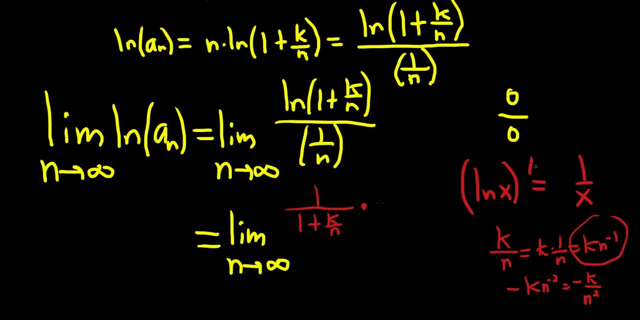 that the derivative of 1 over x is negative. 1 over x squared. in this case it'll be negative k over n, squared. again, you get tired at some point of doing this and you end up just memorizing the derivative of 1 over x. so again it's 1 over whatever is here times the derivative of the. 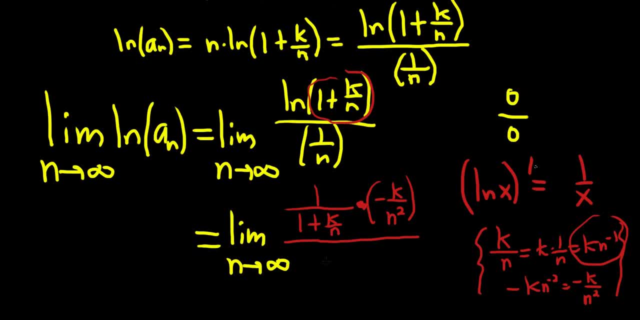 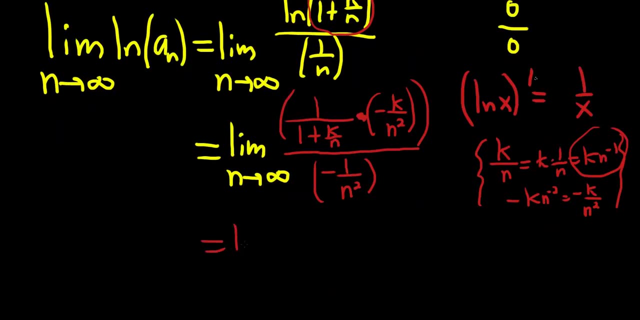 inside over and the bottom. same thing. the derivative of 1 over n is negative, 1 over n, squared right, so you end up memorizing it all right. so we took the derivative of the top, we took the derivative of the bottom, and this is really nice, because some stuff does cancel. this is the limit, as n goes to infinity. 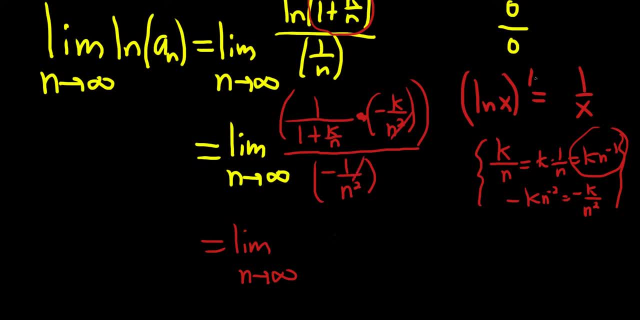 so the negative 1 over n squared cancels with this one. so we're left with negative k over 1 plus k over n. so, oh, oh, the negatives go away. whoops, i messed up right. the negatives cancel. so we're with k, with k over 1 plus k over n. so we're left with negative k over 1 plus k over n. so we're left with. 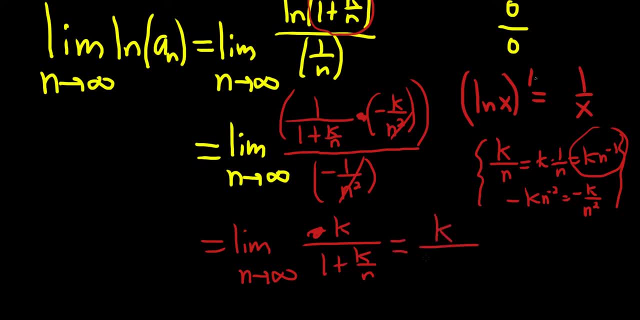 negative k over n, so as n approaches infinity, you get k over 1 plus 0. now we drop the limit sign, so we get k. so we have that the limit of the natural log of a sub n is equal to k. so let's go ahead and. 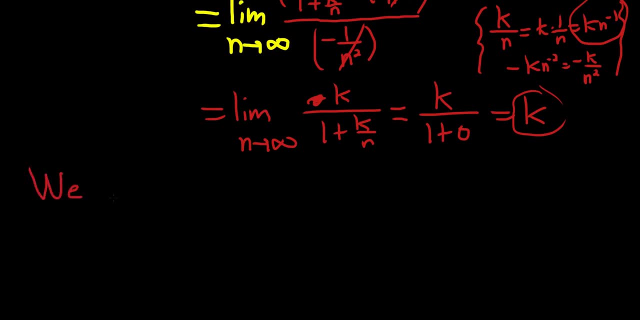 rewrite that. so we showed. we showed that the natural log of a sub n approaches k as n approaches infinity. so we get k over 1 plus 0. now we drop the limit sign, so we get k. so we have n approaches infinity. okay, here's the, here's the punch line. so thus, this is the part that a lot of 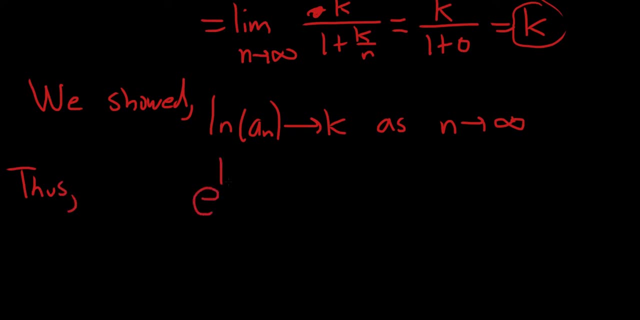 people don't understand e to the natural log of a sub, n approaches e to the k as n approaches infinity. and the reason that this is true- and this is the part that i said that a lot of people don't get, don't think about- is because e to the x is continuous um. so recall the definition of: 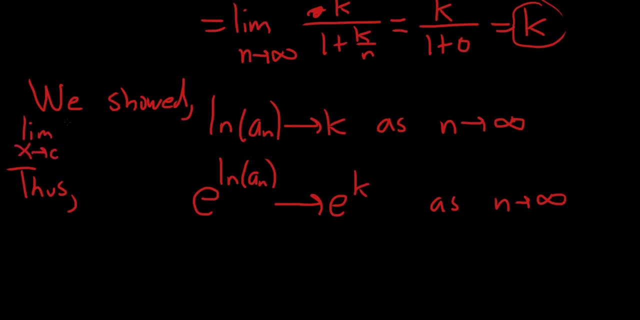 continuity says: if you have the limit as x approaches c of f of x, this is actually equal to f of c. that means you can plug in the number. that's what we're doing here. we're plugging this into the e. we're plugging it into the e.